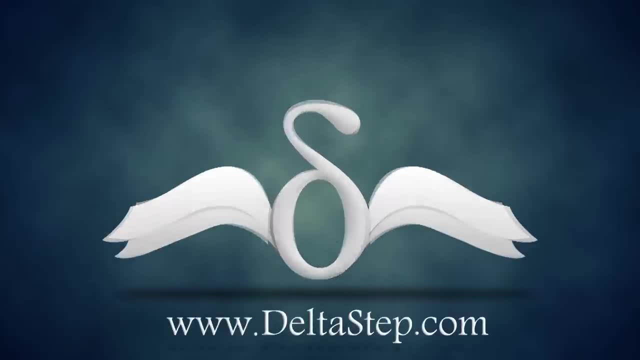 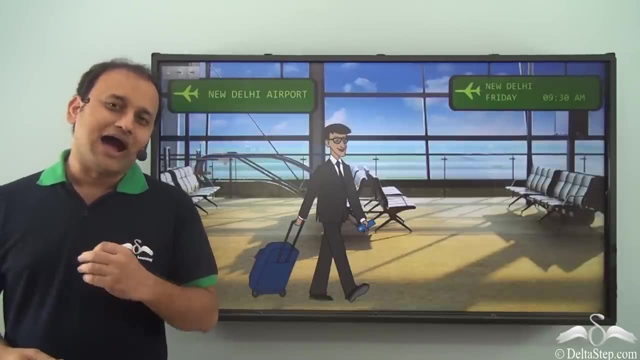 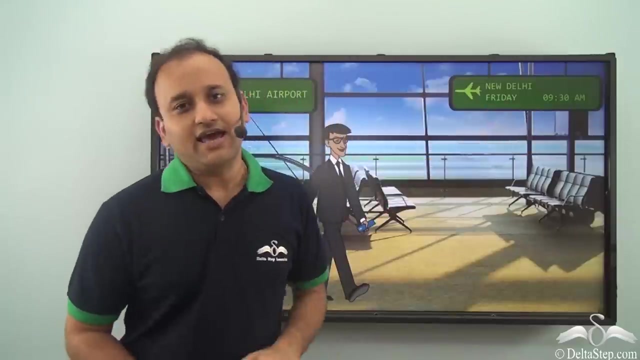 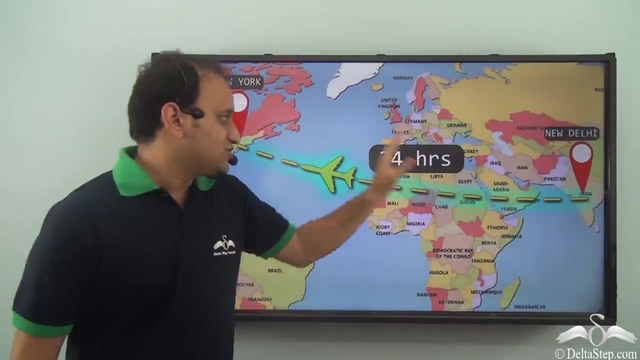 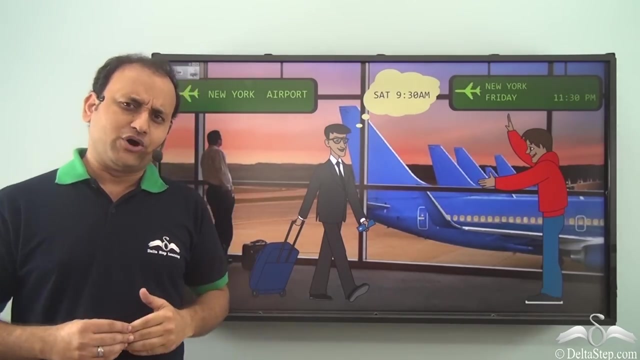 Sam was traveling to New York to meet his best friend, Amar Now. his flight left New Delhi Airport on Friday 9.30 am Now. his flight took exactly 24 hours to reach New York from Delhi. Now, once he reached New York he was pretty sure that he left. 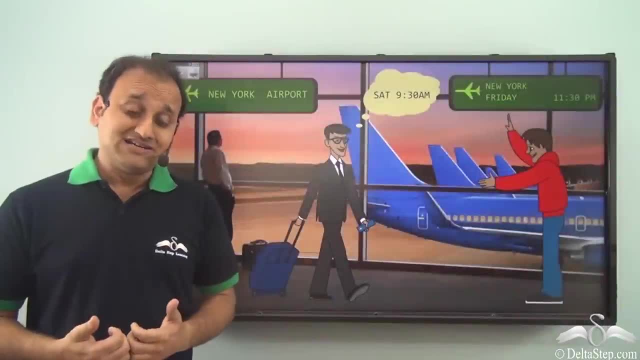 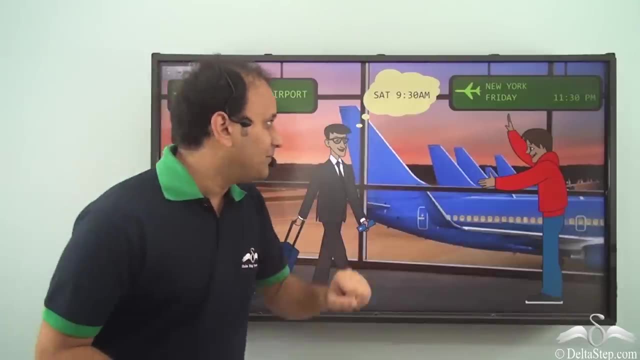 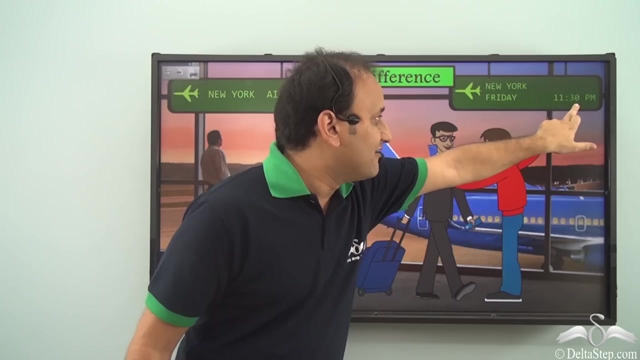 Delhi at 9.30 am Friday. So after 24 hours it is definitely 9.30 am Saturday in New York. But when he met Amar, Amar showed him the clock and on the clock it was till 11.30 pm Friday. 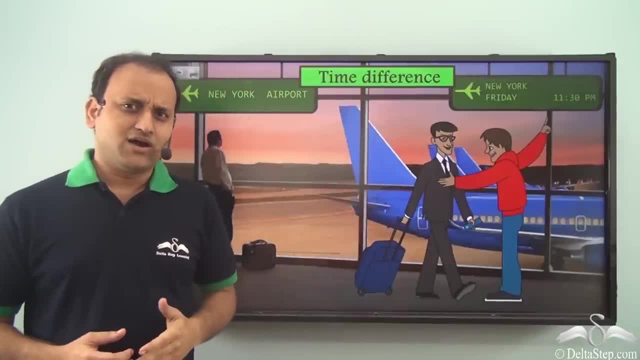 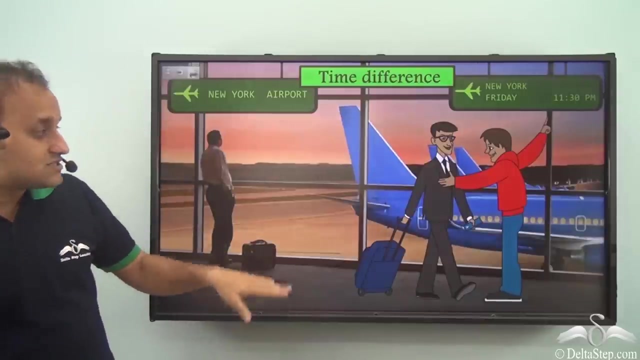 So Sam was very amazed. How can that happen? He left at 9.30 am Friday and it took him 24 hours to reach New York, and still the time is till 11.30 pm Friday in New York. Well, that's because New York and New Delhi followed different time. 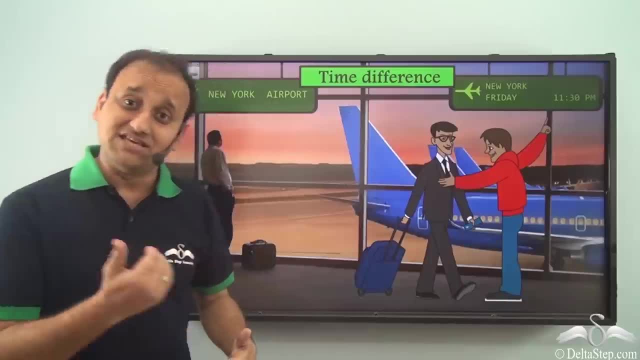 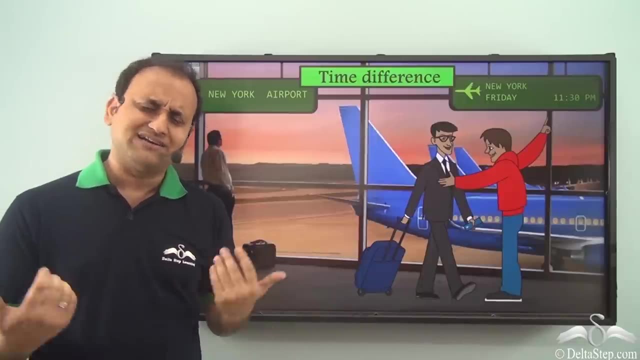 zones, That is, there is a time difference between these two cities. Now you must be wondering: why do they have different time zones or why do they have different times? They can have a single time all around the world. It would be much convenient, isn't? 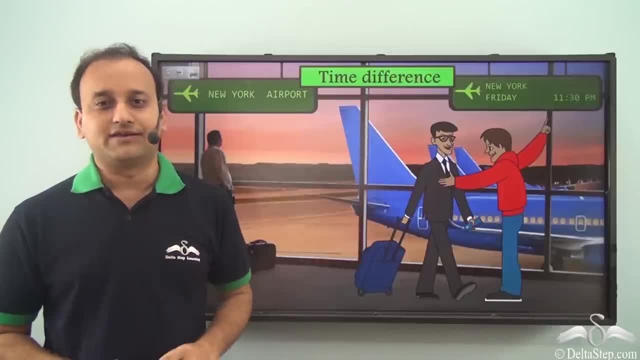 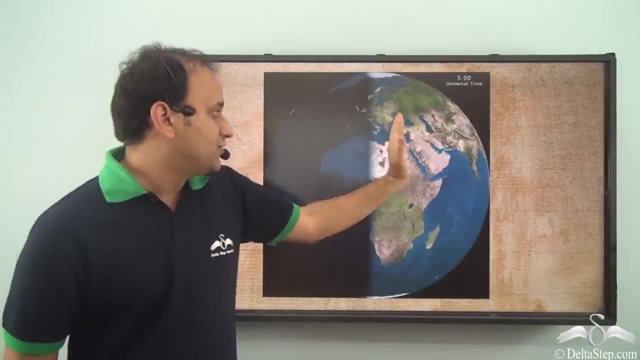 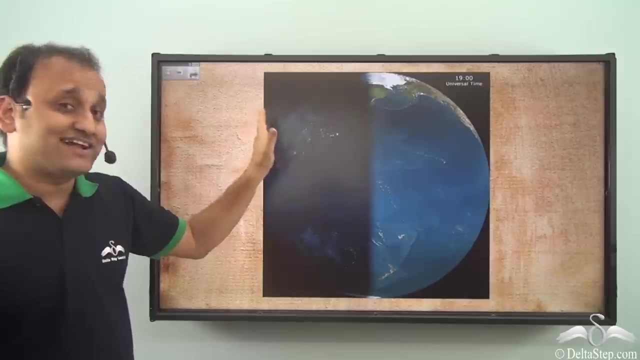 it Calculating the time, But there is a reason behind it. I'll show you why. Now, this is how the earth rotates continuously. So, as you can see, all the places on the earth do not have day and night at the same time. So, while 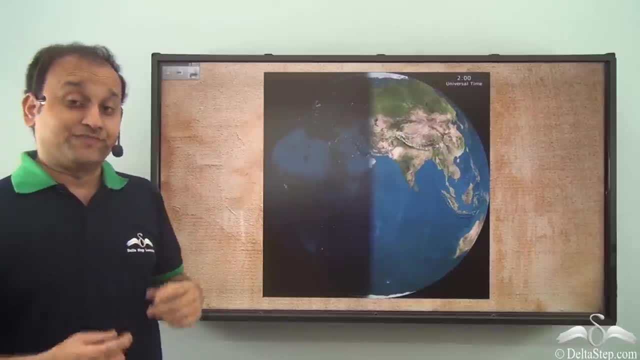 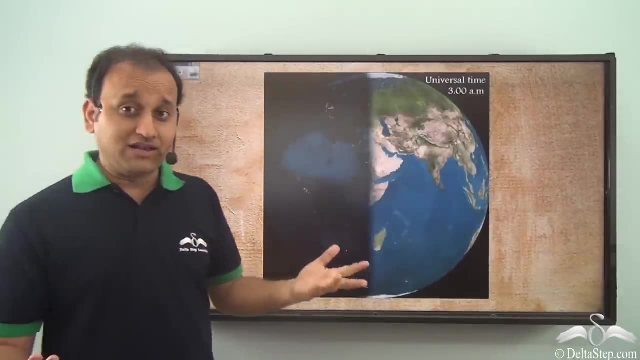 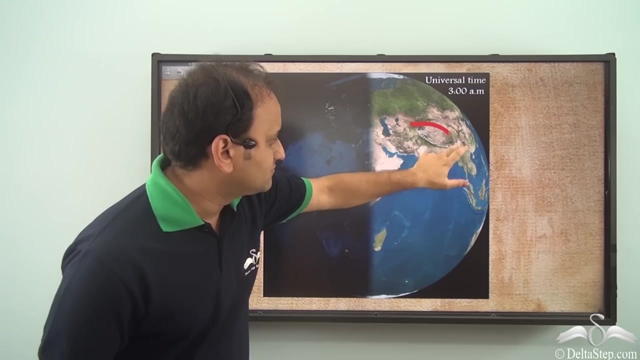 some places have day, others have night. Now, if all of them followed the same time, what would happen? Well, for example, if we have a universal time, Now, at 3am, it is broad daylight in India. as you can see here, it is broad daylight. 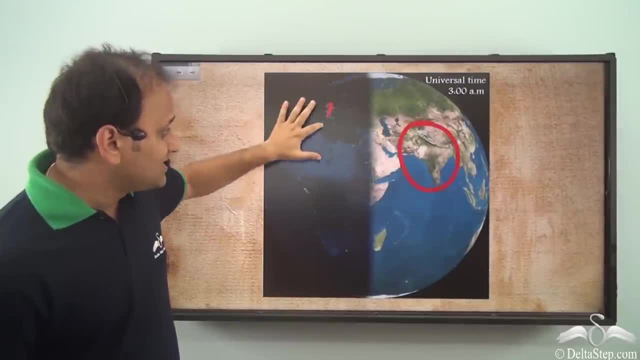 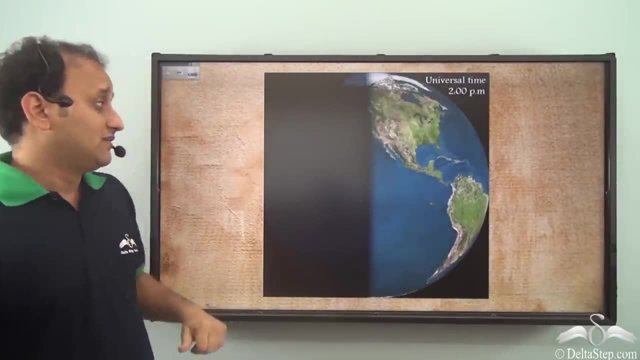 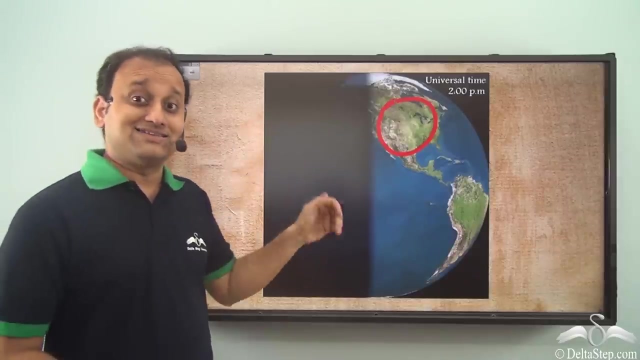 and, at the same time, it is night in this portion of the world. Now, what happens when it is 2 pm? Well, when it's 2 pm, it's broad daylight in America, while India is in darkness, That is, it is night time. So how would you feel if 2 pm is night and 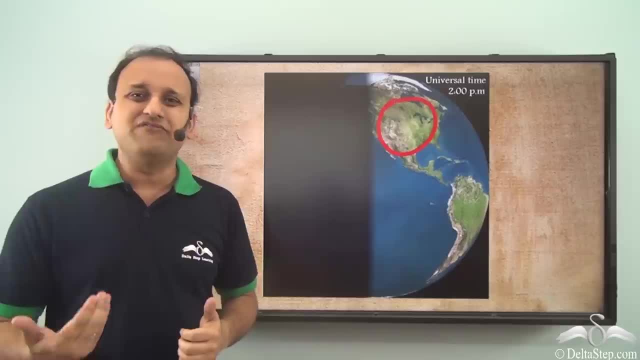 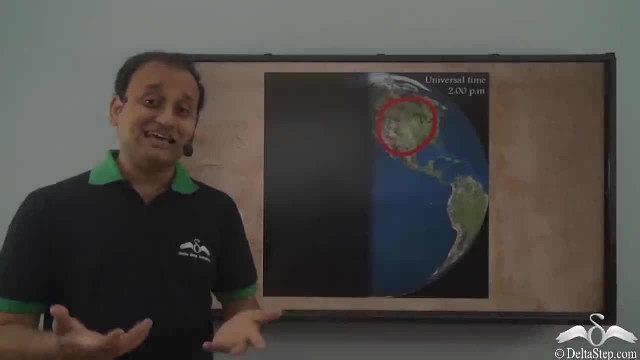 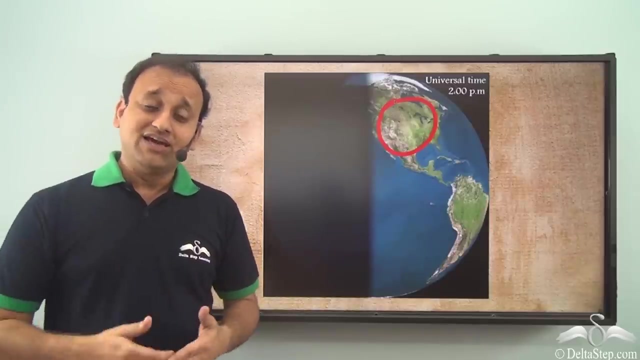 3 am is suddenly broad daylight. for you. It will be very inconvenient, isn't it? So we follow time according to movement of the earth. That is, in the day time we have 11 am or 1 pm, 2 pm and so on, and after 5 pm usually we have evenings and then 11. 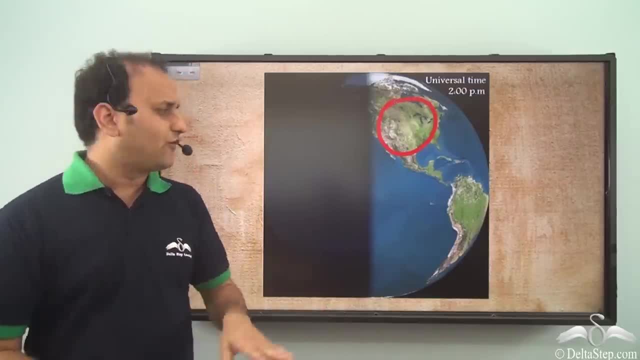 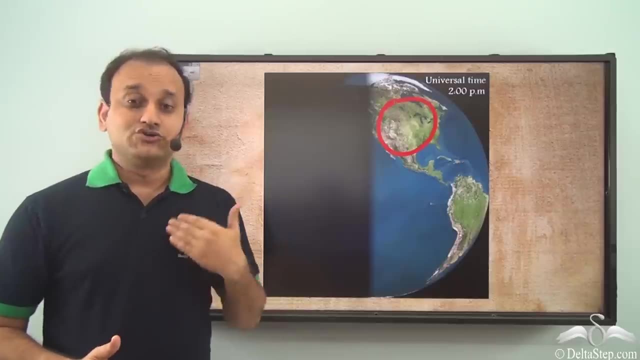 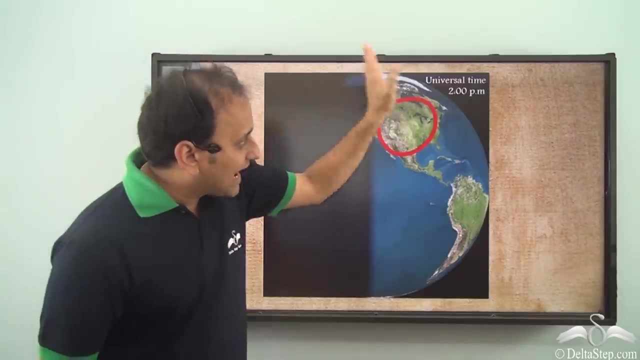 pm is night for us. Now, this is a schedule which is followed by all the different places on earth, and that is why they have different time zones, so that, according to their day time and night time, they will have their clock running, and that is why we have time difference. 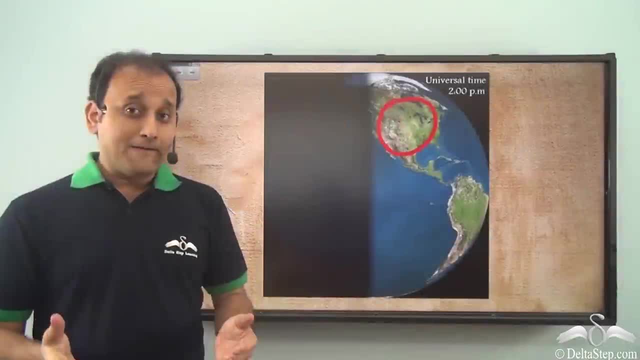 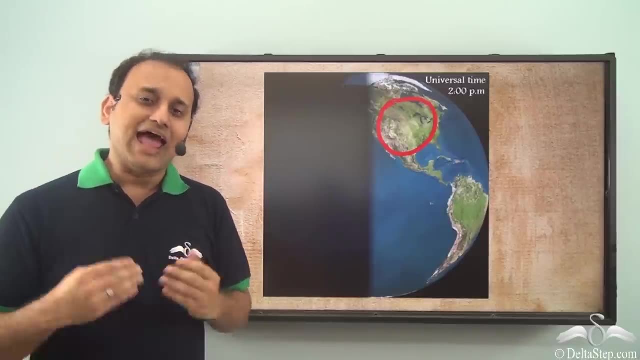 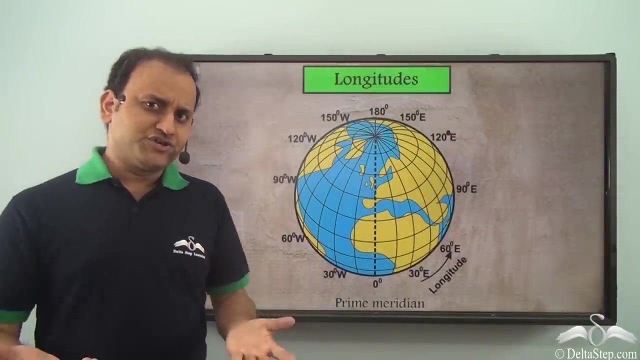 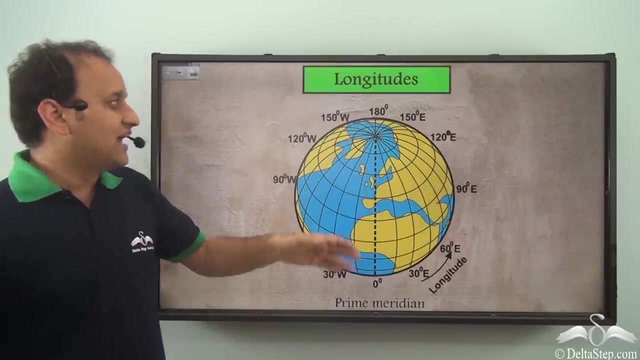 between different places on the earth. So, because of the rotation of the earth, as we saw, different places have day and night at different times. As a result, they follow different time zones. Now the question arises: how do we decide which place follows what time zone? Well, that is done with the help of these imaginary 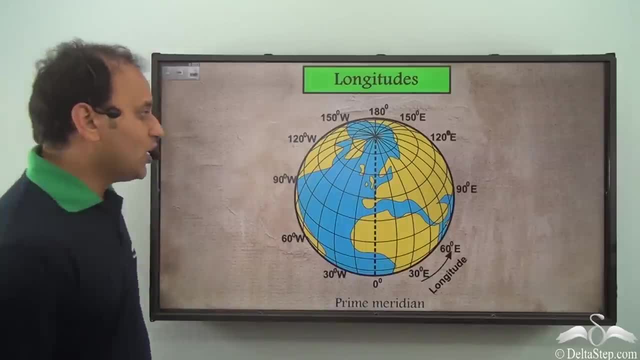 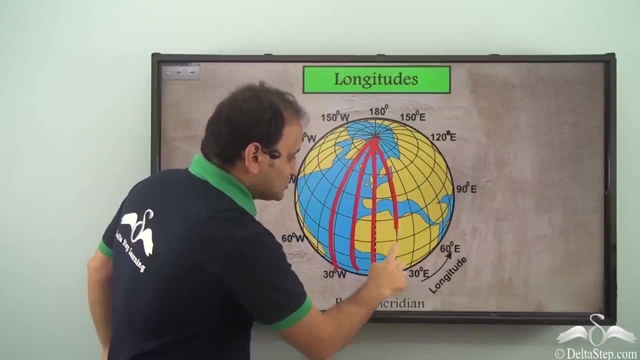 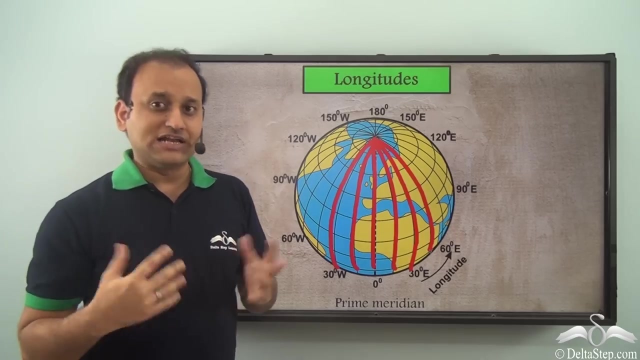 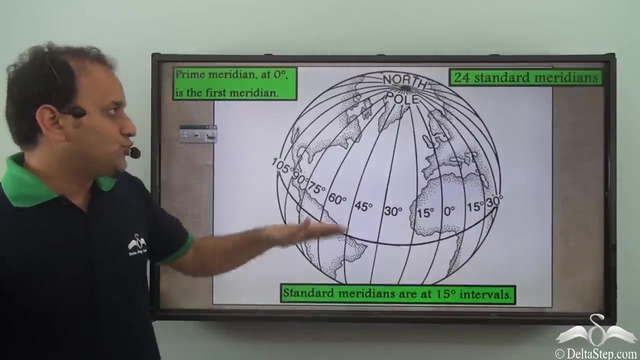 lines on the earth's surface, which are called longitudes. So all these lines here, these all lines decide which country will follow which time zone. So let's understand how that works. So we see here, among all the different longitudes, 24 has been marked as. 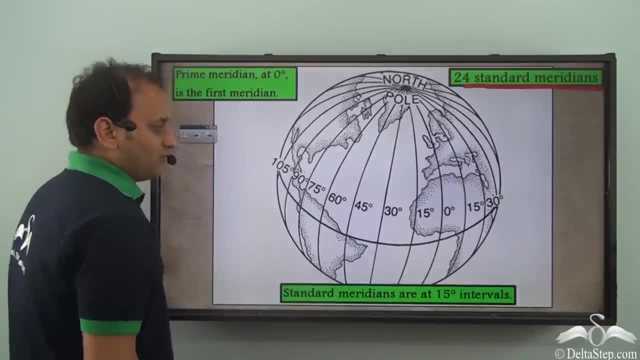 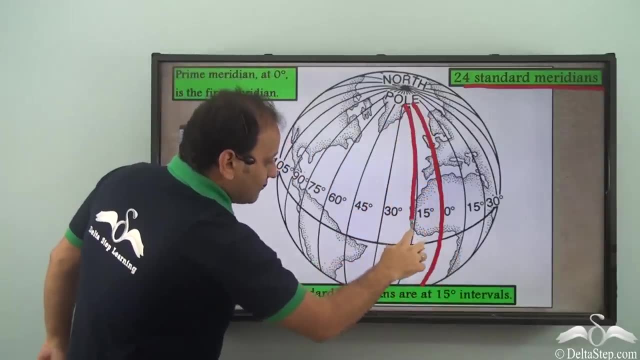 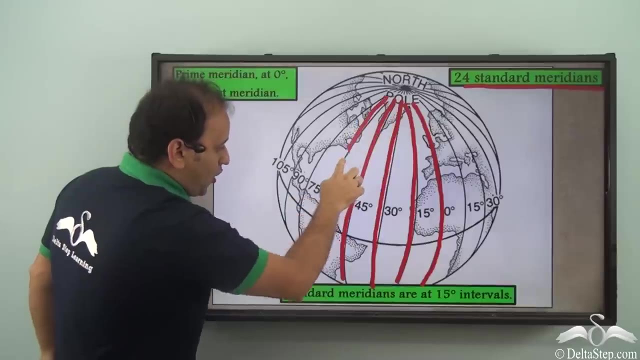 standard meridians. Now, what are the standard meridians? Well, if you take prime meridian as 0 degree, then the longitudes at 15 degree intervals are called standard meridians. So you see, all these lines are standard meridians. 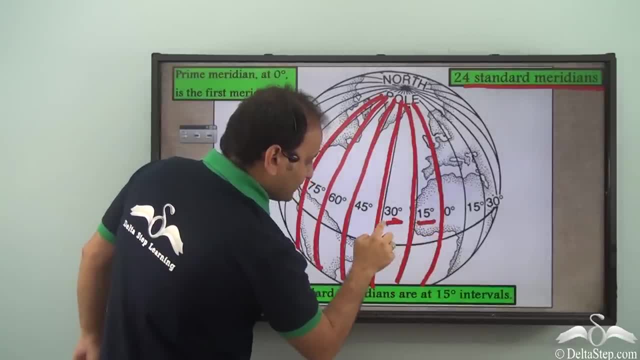 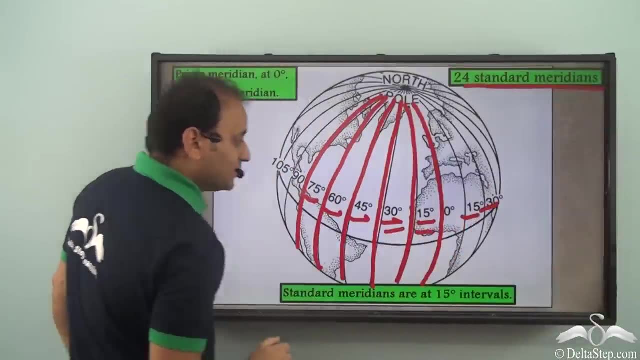 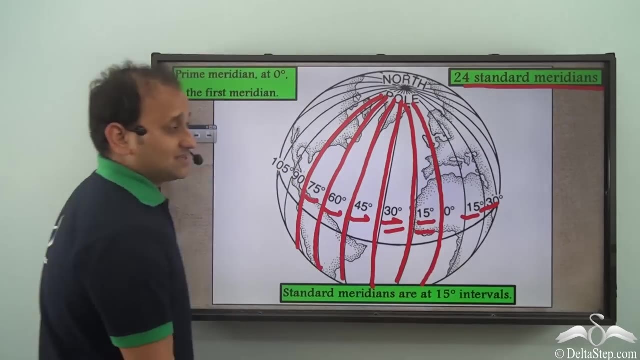 and, as you will notice, the difference between them is always 15 degrees. So, on east as well as west of the prime meridian, we have meridians at 15 degree intervals, which are called standard meridians, and there are total of 24 standard meridians on the planet earth. 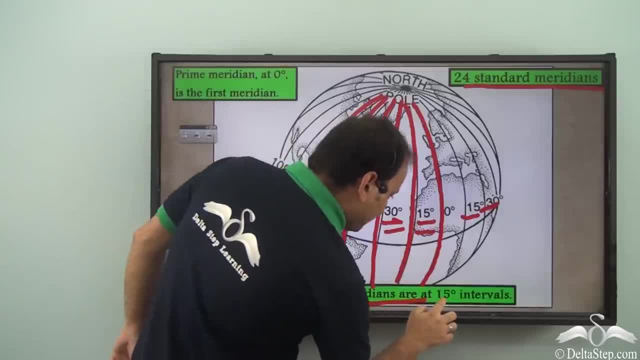 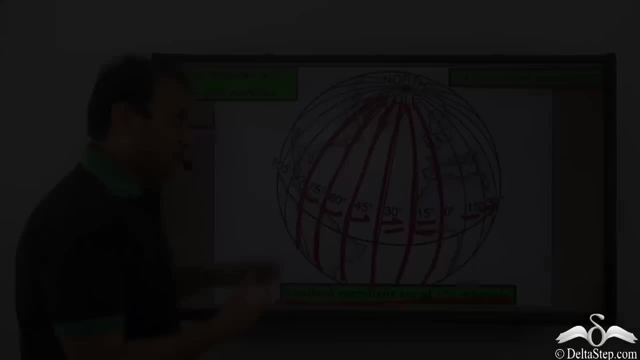 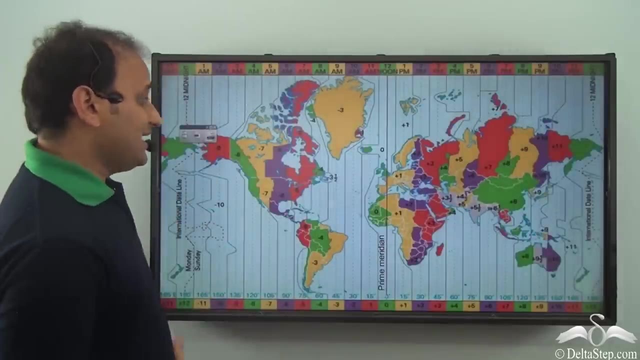 So standard meridians are at 15 degree intervals. Now, how do they help us in deciding the time zone? Well, if we flatten this thing on a piece of paper for easier understanding, it will look something like this: Now, what do we see here? Well, 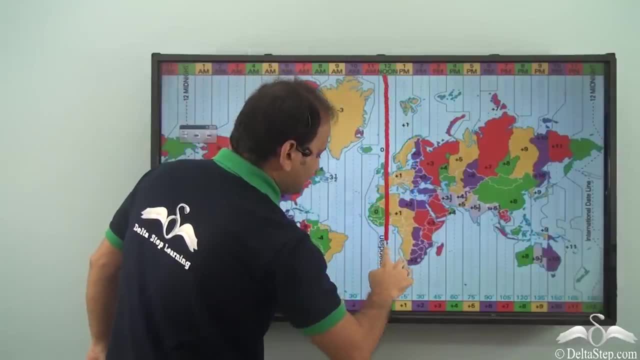 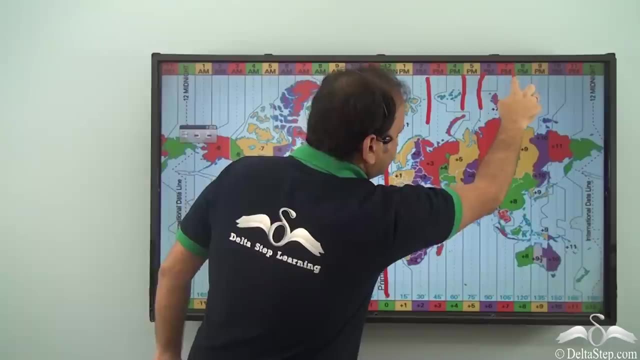 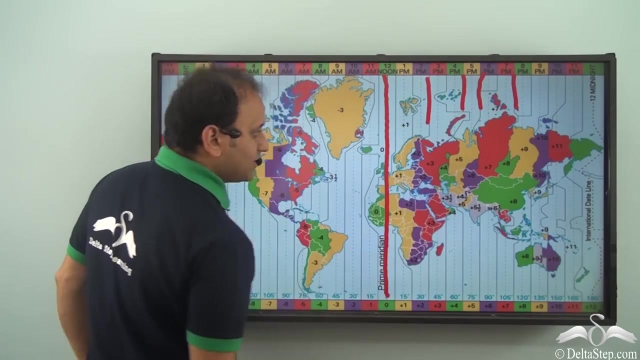 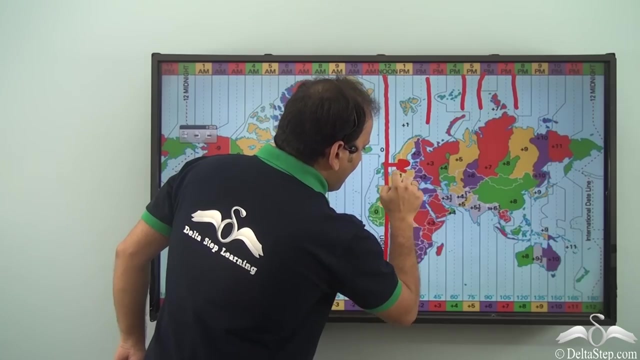 this is the prime meridian and all these lines here, these are the standard meridians. So how do they decide time? Well, as you move eastwards from the prime meridian, with every standard meridian we have an addition of one hour in the time. So if it is 12 noon at prime meridian, 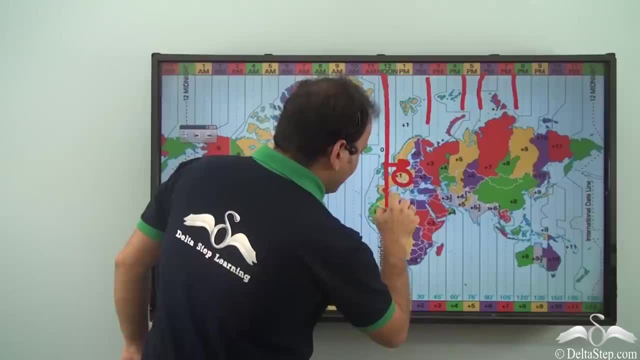 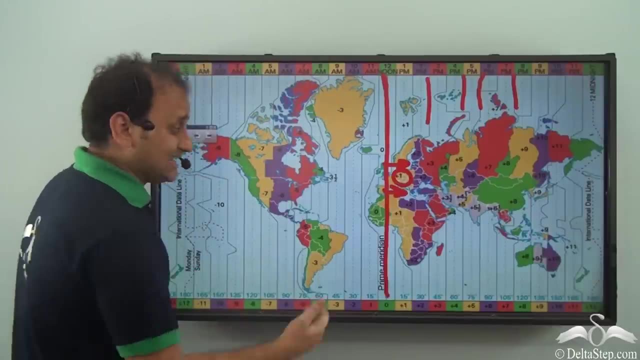 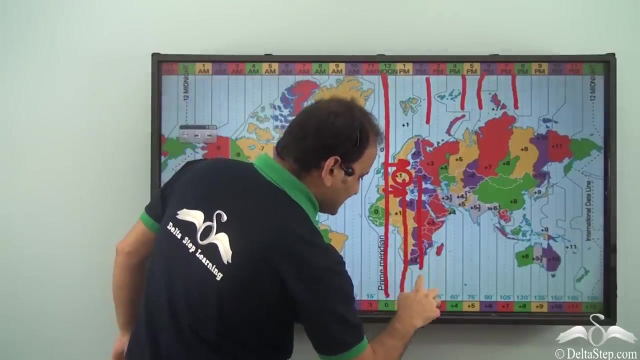 then when we go towards the first standard meridian on the east, so plus one hour, that is, it will be 1 pm in this area and then it will be 2 pm in this area, and so on, it will keep on increasing Plus one hour. 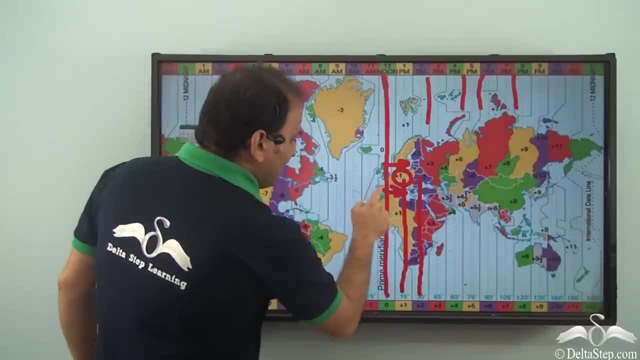 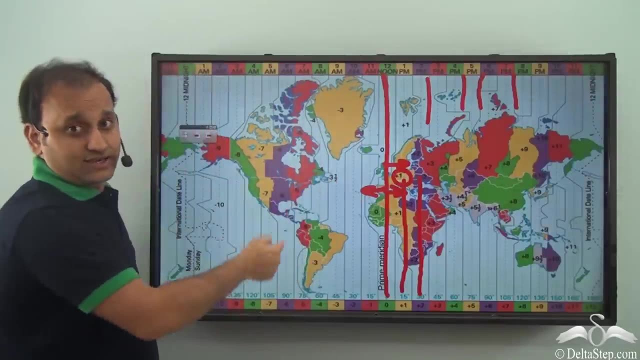 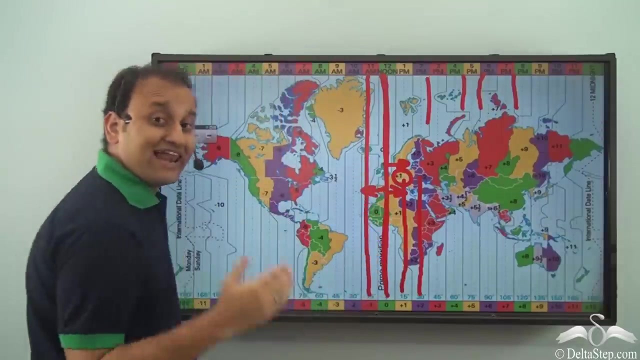 for each standard meridian. Similarly, when we move westwards, then for every standard meridian one hour is decreasing. So if it is 12 noon here, then for the first standard meridian this area will have 11 am, and then similarly. 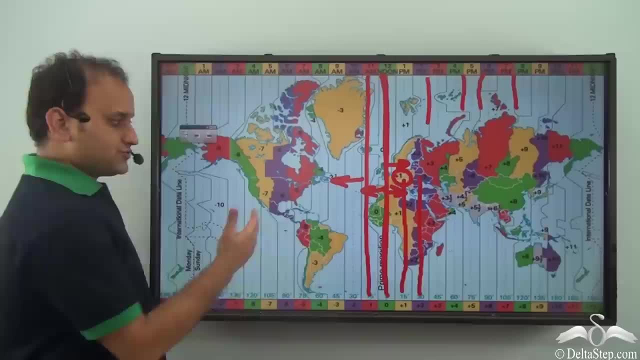 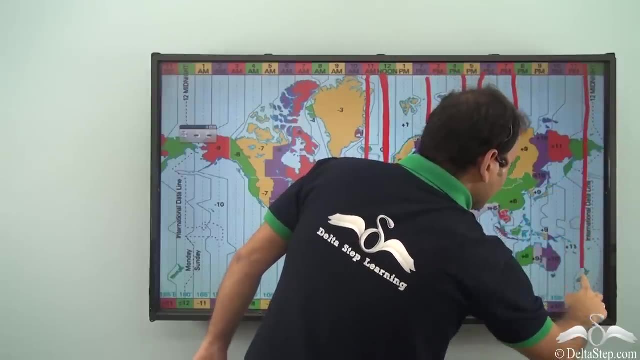 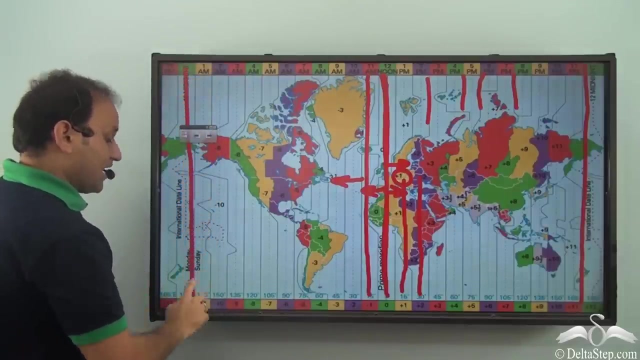 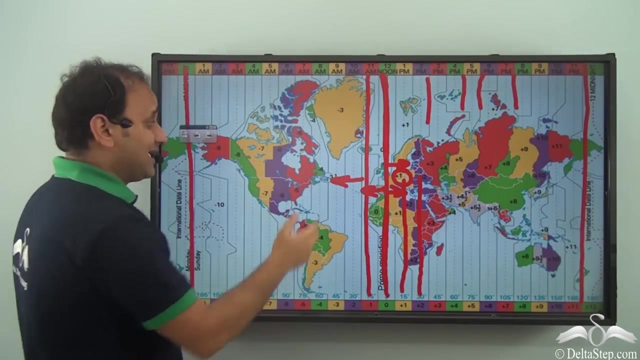 one hour will keep on decreasing. So, if you notice, the eastmost point here and the westmost point here have completely opposite timings. This place is 12 hours ahead of the prime meridian and this place is 12 hours behind the prime meridian. 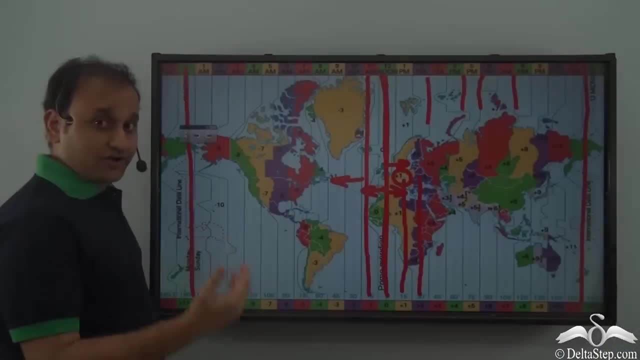 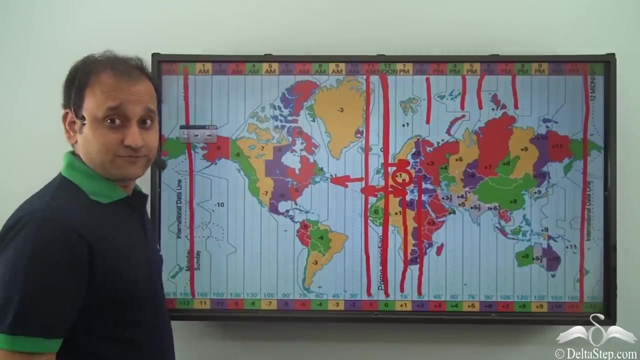 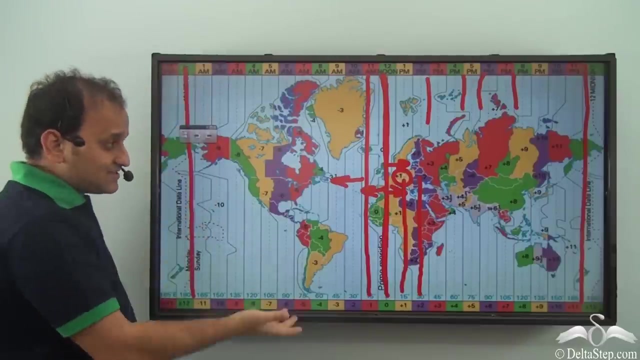 Now, why is that? Well, that's because our earth rotates from west to east, So the easternmost place will have morning first, and as we move towards the west, they will have morning later and, as a result, these places are 12 hours ahead of the prime meridian. and these are: 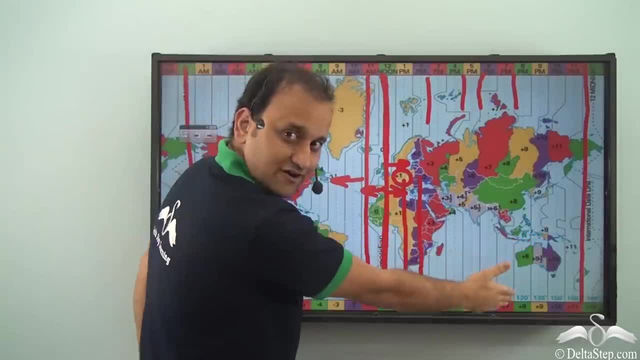 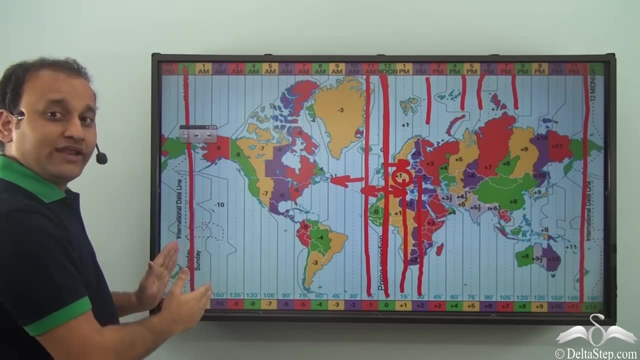 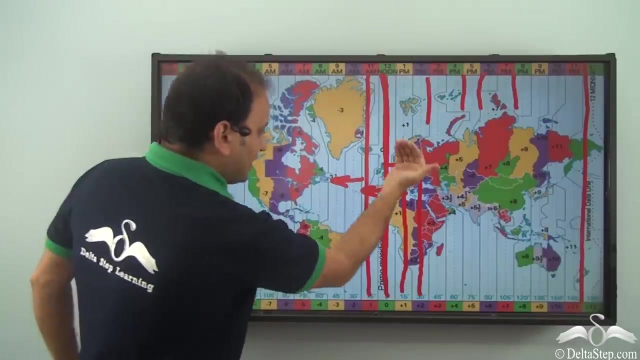 behind the prime meridian, because they will face the sun first, they will have mornings first, and slowly, as you move towards west, this place will finally have the morning when already that place will have night. So as the Earth rotates, so different places have different time zones, so that 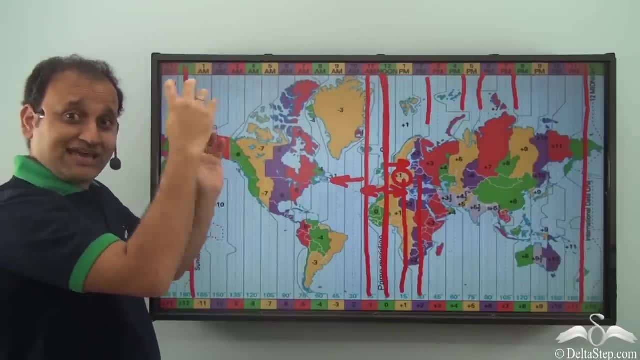 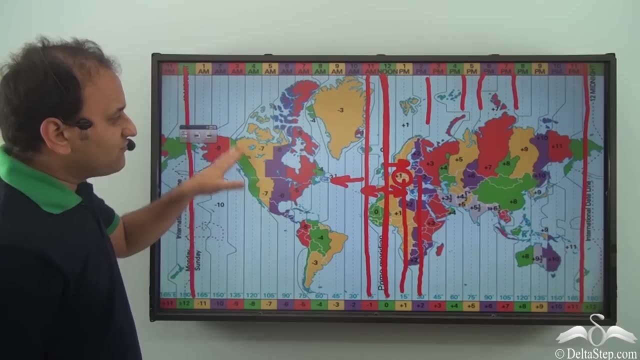 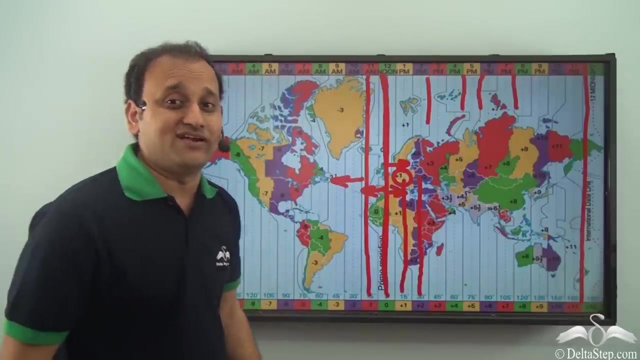 as the earth rotates, the sun's position is changing for them and, as a result, their clock's position is also changing accordingly, and that's why we have so many different time zones, and all these time zones are decided by the standard meridians. So from the prime meridian if you move east, 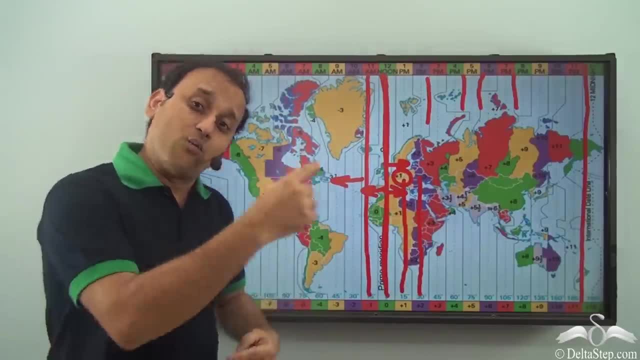 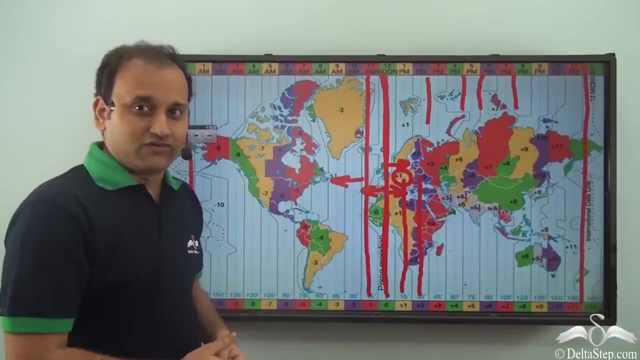 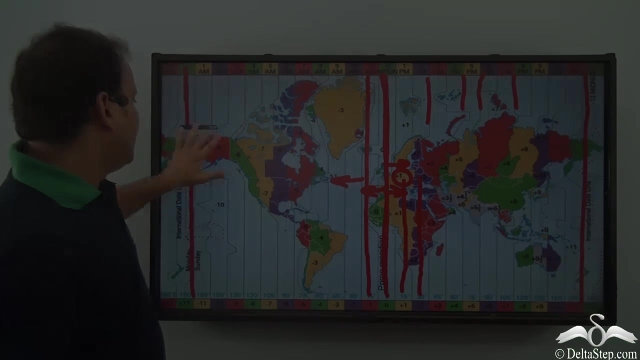 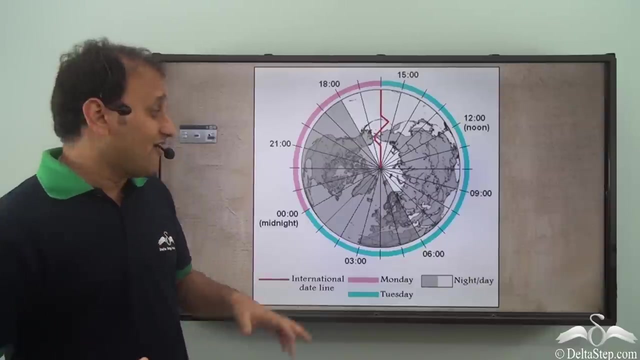 words: for every standard meridian, we add one hour, and if you move westwards, for every standard meridian we deduct one hour, and this is how the time zone of the entire earth is managed. Now I will share with you a very interesting fact Now: how time zones can really be a very interesting thing to know. For example, 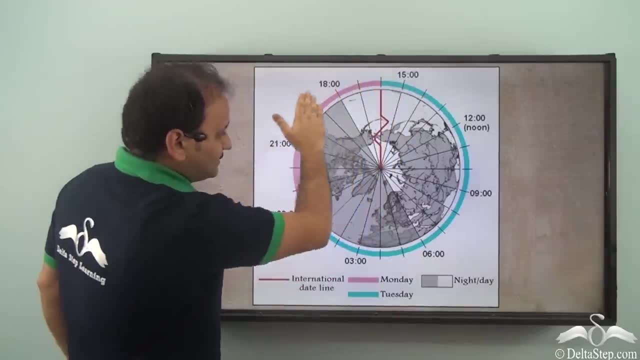 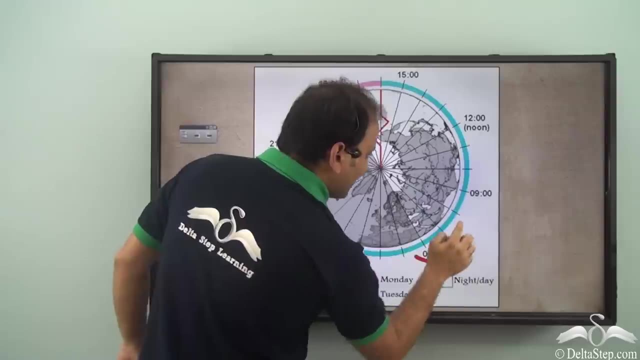 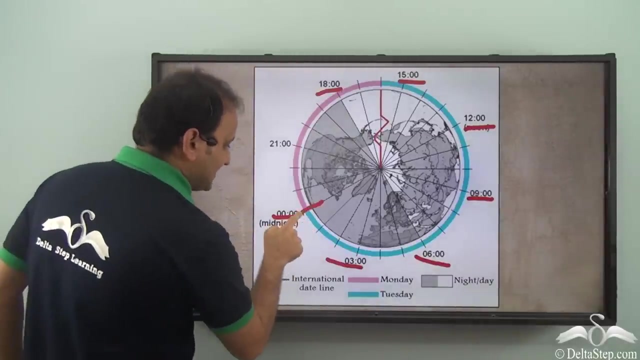 what do you see here? Well, the entire earth has been divided into different time zones, and according to time zones, we have times at different places in the world. So what happens at this point in time At this place? it is midnight, isn't it? Now, all these places are currently. 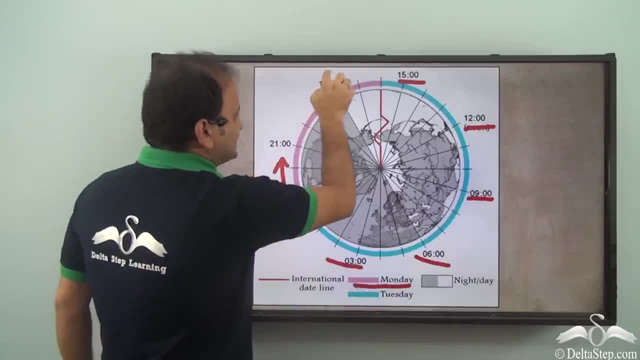 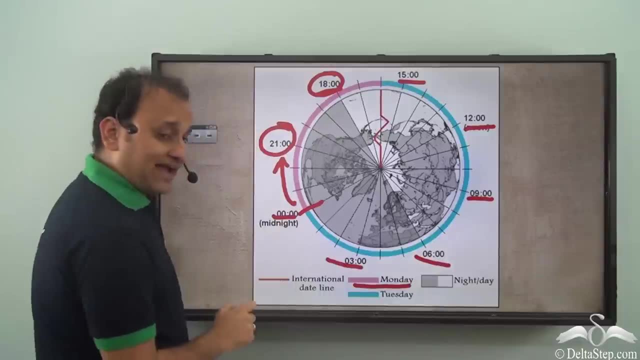 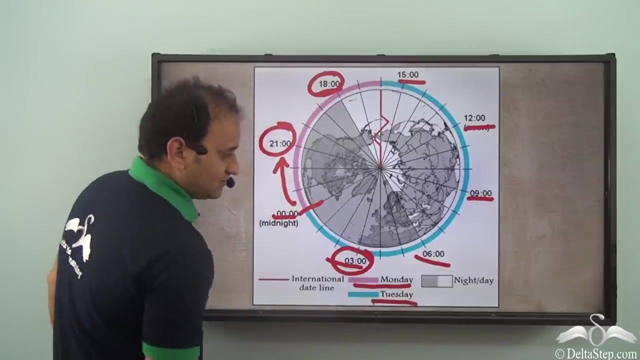 having Monday. So it is Monday 6 pm at this place, Monday 9 pm at this place, while once you cross the midnight the day would change. So this place has 3 am on Tuesday. this place has 6 am on Tuesday. this place has 9 am on. 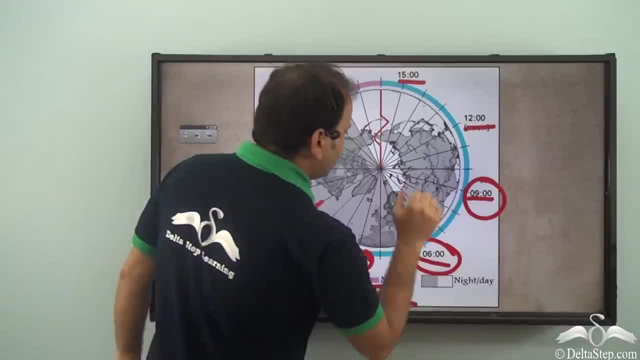 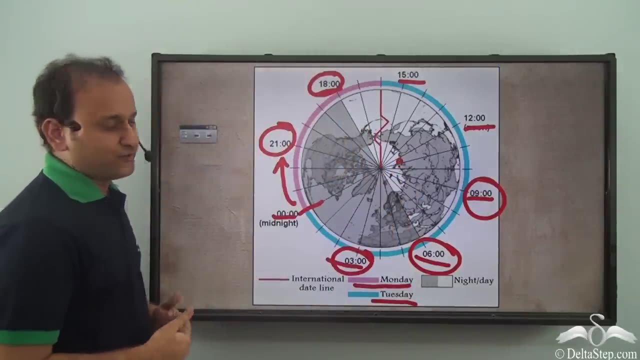 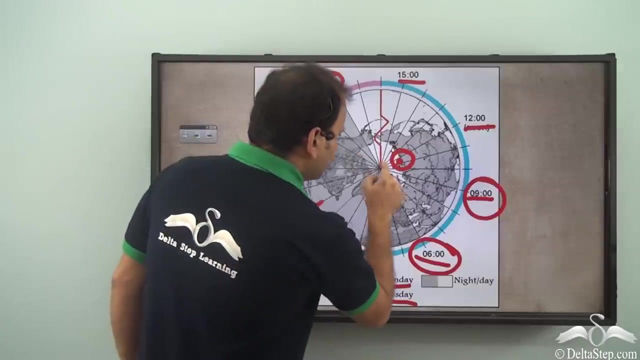 Tuesday and so on. Now, if you are living somewhere here. so what's the time, What is the local time for you? So it's around 11 am for you when you are living here. Now, if you start traveling from here, take a flight. 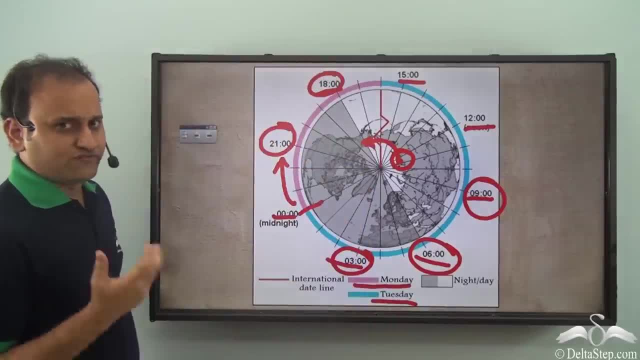 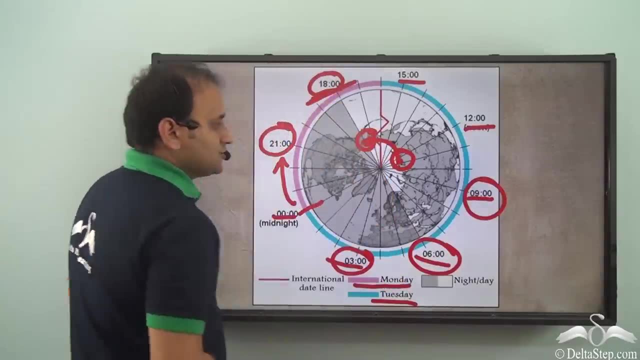 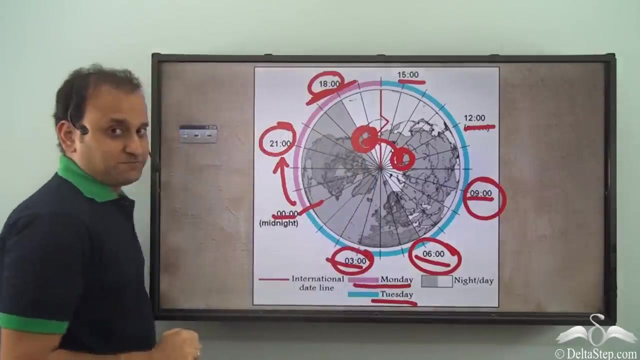 and reach here, Then what will be the time? The local time? It will be 6 pm, isn't it, As you can see here? So you were here and is 11 am. now you have come here and it is 6. 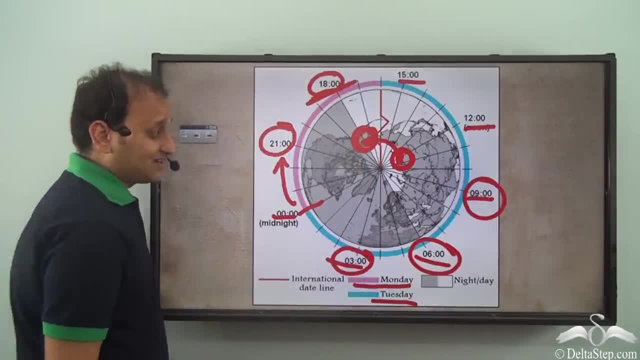 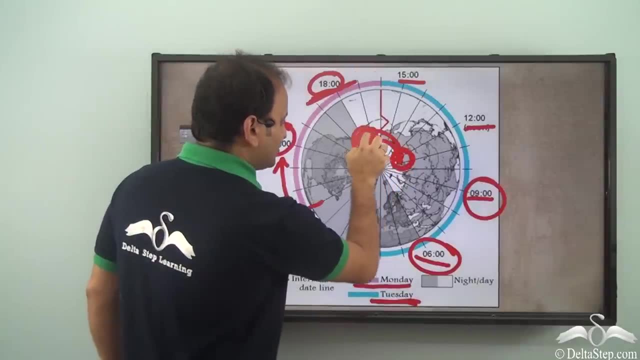 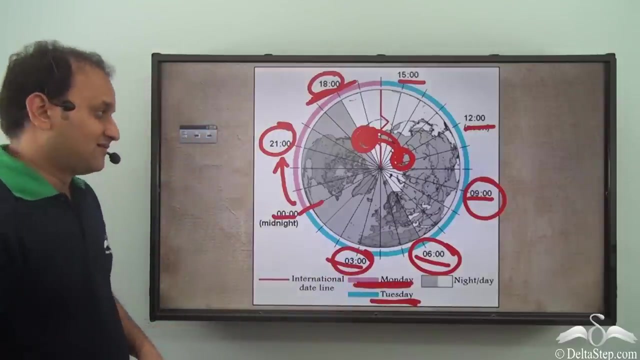 pm. but another interesting fact is that here the 11 am is what It is: Tuesday 11 am, and as you travel from here to here, now it is Monday 6 pm, Monday 6 pm. So what exactly happened? Once you travel from here to here, the date changed. 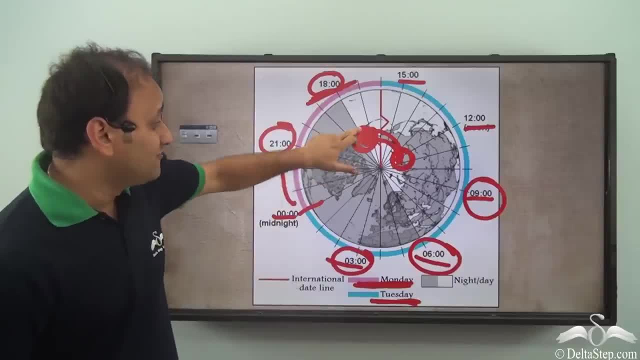 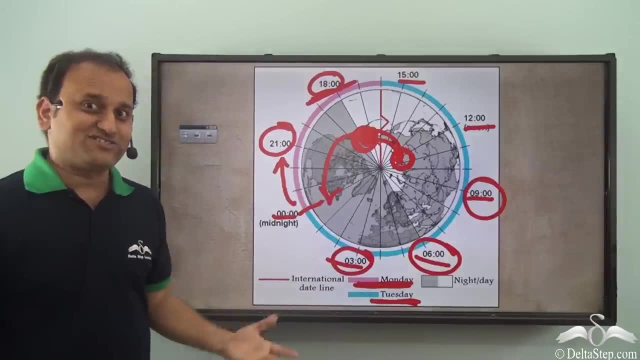 You went back in time, So you will be able to live the entire evening of Monday once again. This is the interesting thing about time zone. So when you are traveling from one time zone to the other, you are gaining time, or if you travel from here to here, you 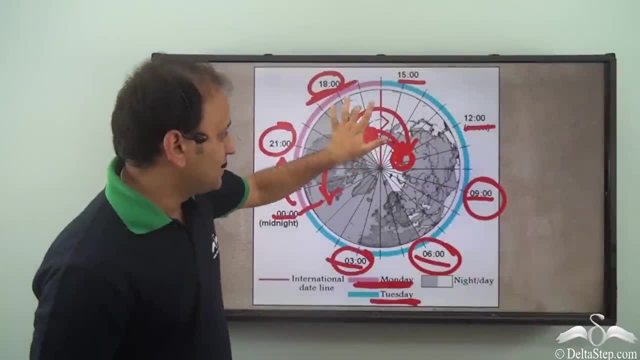 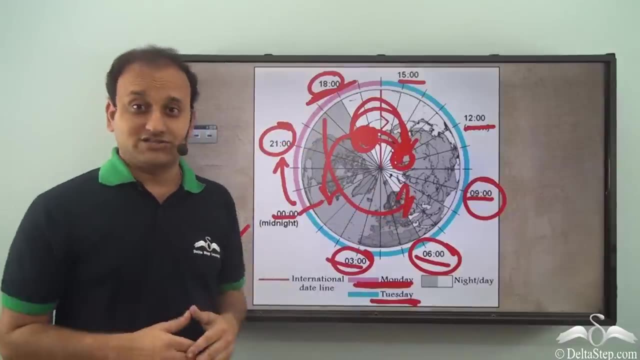 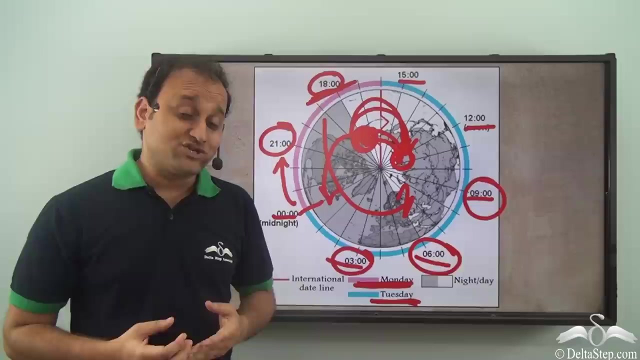 are losing time because from Monday 6 pm you suddenly come to Tuesday 11 am, So all the time in between is lost. So this is a very interesting thing about time zone. So if you are able to travel efficiently, you can actually gain time or lose time, according. 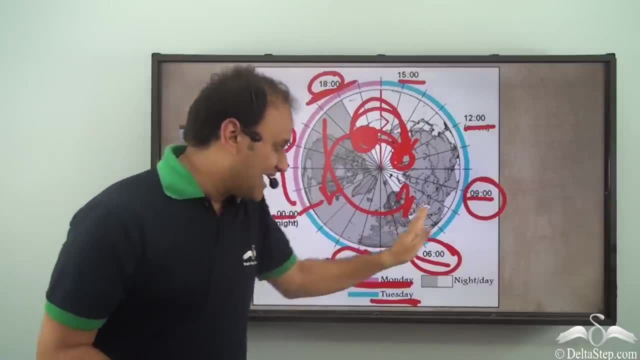 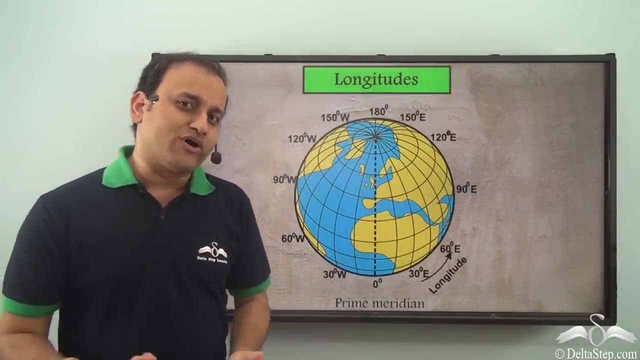 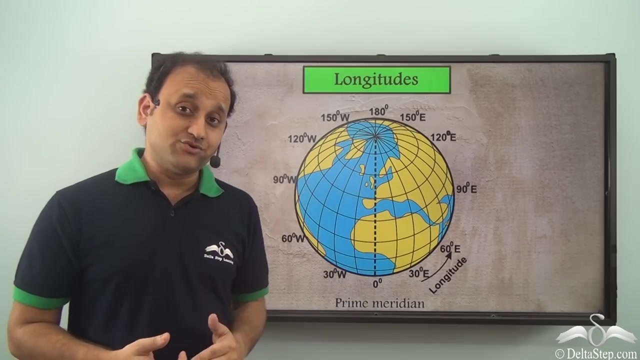 to your liking, And that's how the time zone works. So you see, longitudes are the very important lines on planet earth, because they definitely help you locate a place, along with latitudes. At the same time, they divide the entire earth into a number of time zones. 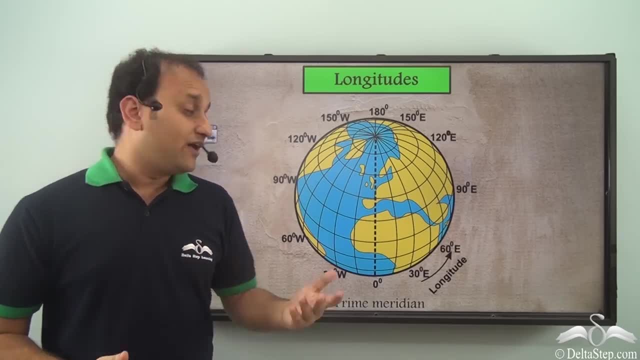 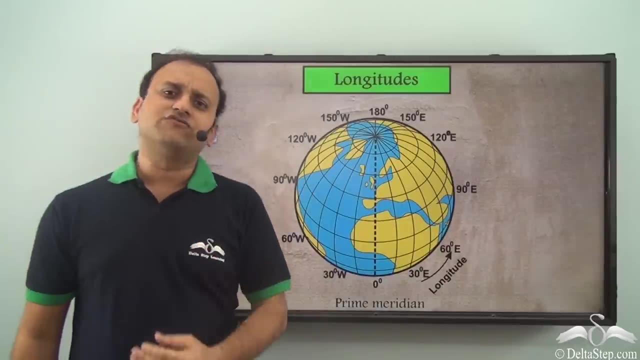 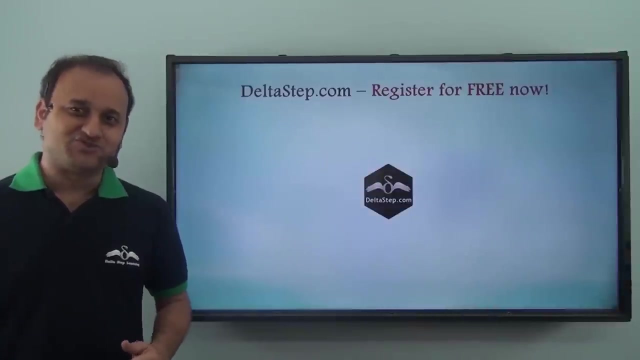 so that we all can have practical times where we can manage our times according to our day and night. And so longitudes are one of the very important imaginary lines for all of us. Don't forget to subscribe to our channel. You can also register for free at deltastepcom.